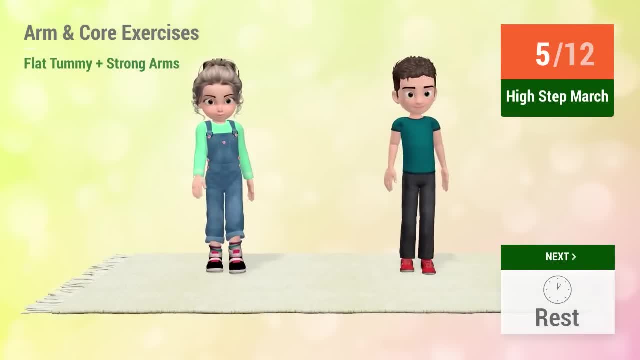 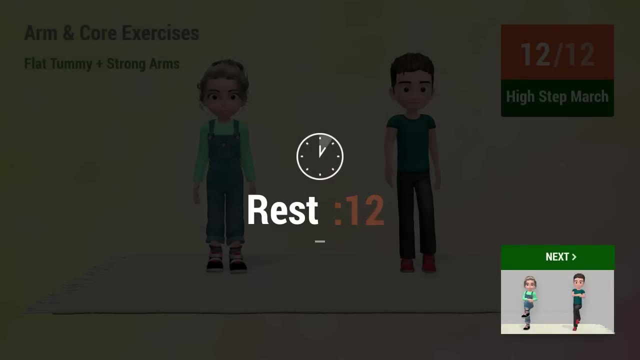 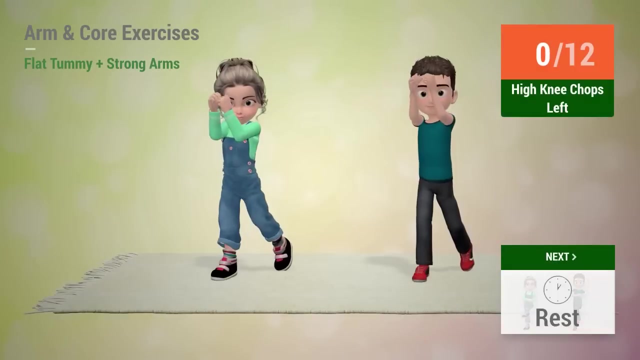 Rest time 3,, 4,, 5,, 6,, 7,, 8,, 9,, 10,, 11,, 12.. Rest time Up next: high knee chops In 5,, 4,, 3,, 2,, 1, go. 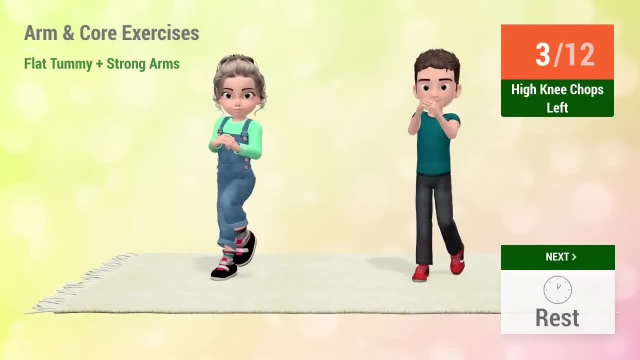 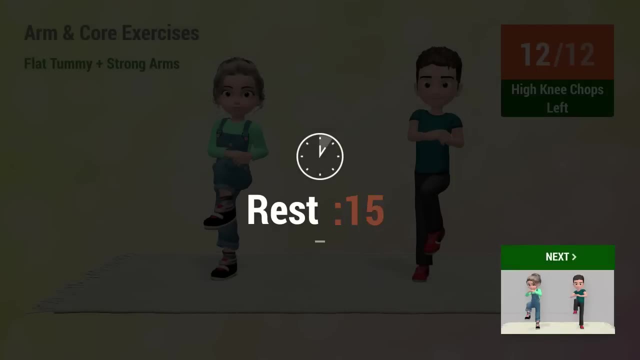 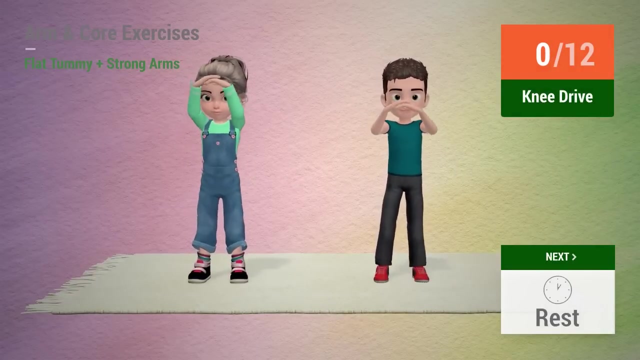 1,, 2,, 3,, 4,, 5,, 6,, 7,, 8,, 9,, 10,, 11,, 12.. Rest time: Up next knee: drive In 5,, 4,, 3,, 2,, 1, go. 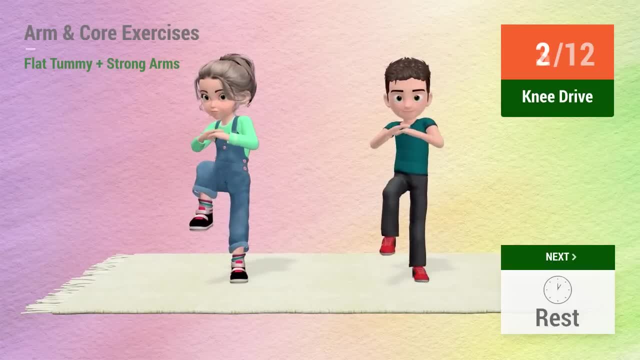 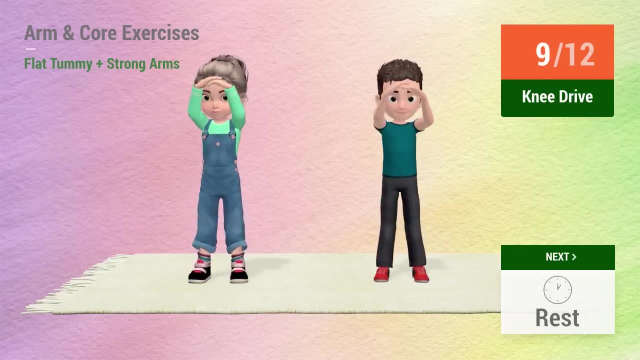 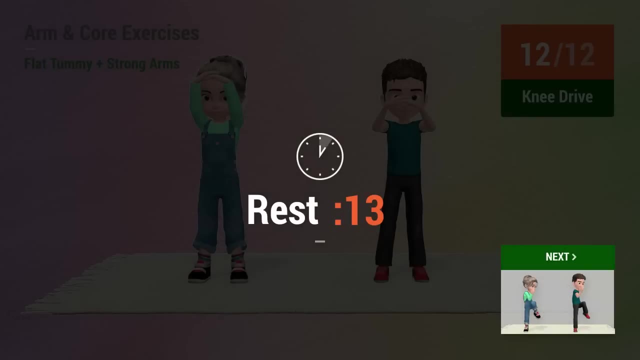 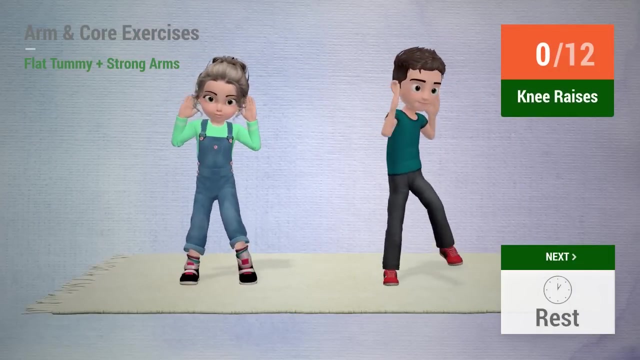 1,, 2,, 3,, 4,, 5,, 6,, 7,, 8,, 9,, 10,, 11, 12 Rest time. Up next knee raises In 5,, 4,, 3,, 2,, 1, go. 1,, 2,, 3,, 4,, 5,, 6,, 7,, 8,, 9,, 10,, 11, 12. Rest time: 1,, 2,, 3,, 4,, 5,, 6,, 7,, 8,, 9,, 10,, 11, 12. 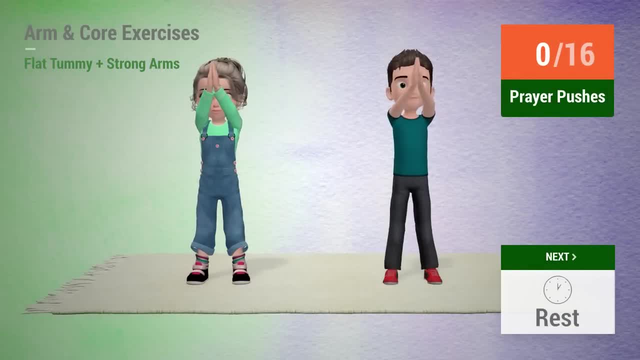 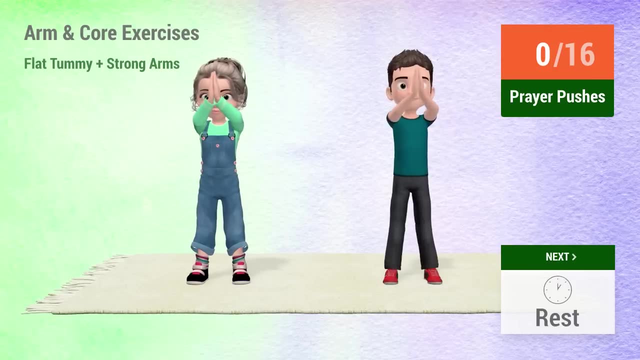 Up. next prayer pushes In: 5,, 4,, 3,, 2,, 1, go 1,, 2,, 3,, 4,, 5,, 6,, 7,, 8,, 9,, 10,, 11,, 12. 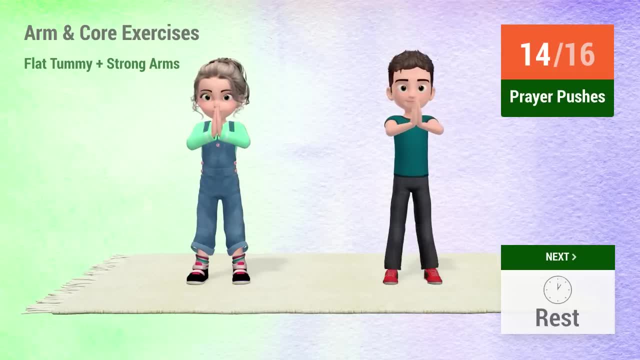 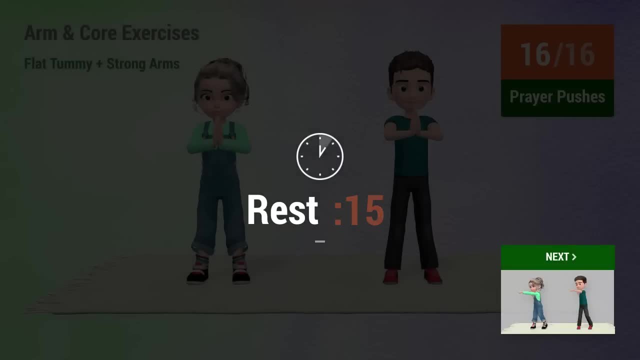 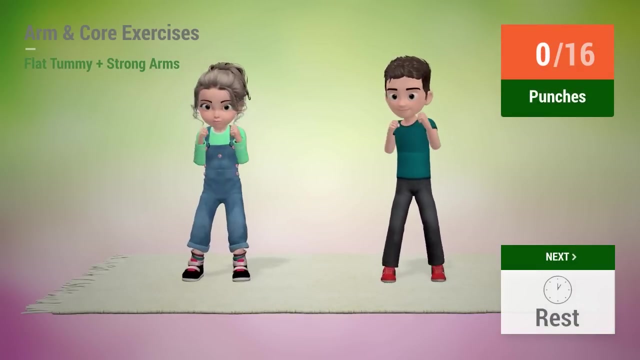 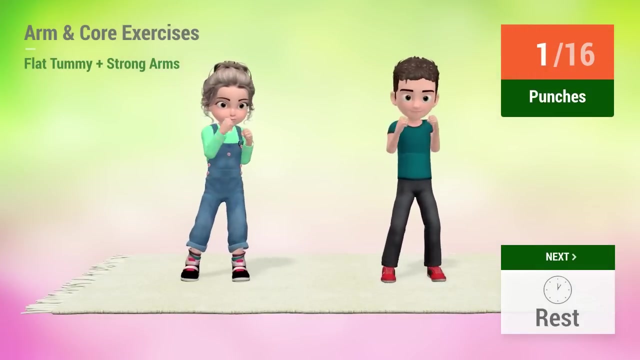 13,, 14,, 15, 16. Rest time. Up next punches In: 5,, 4,, 3,, 2, 1, go 1, 2,, 3,, 4,, 5,, 6,, 7,, 8,, 9,, 10,, 11,, 12,, 13,, 14,, 15, 16. 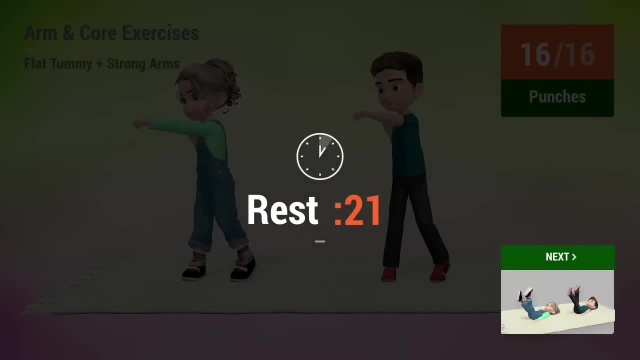 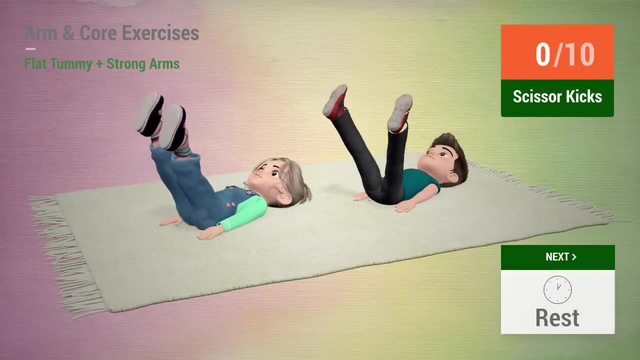 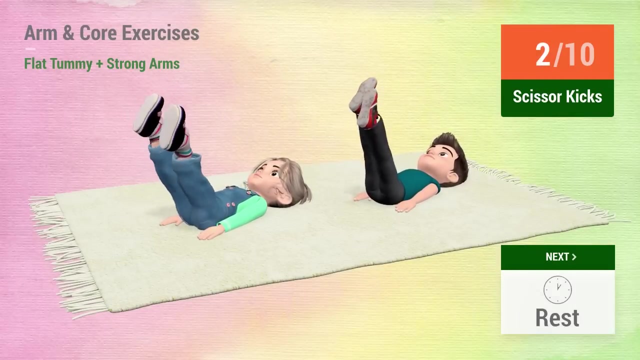 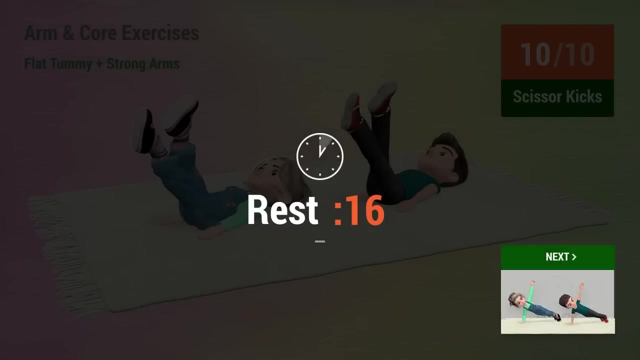 Rest time. Rest time. Up next, scissor kicks In 5,, 4,, 3,, 2, 1,. go In 5,, 4,, 3,, 2, 1,. go 1, 2,, 3,, 4,, 5,, 6,, 7,, 8,, 9, 10. 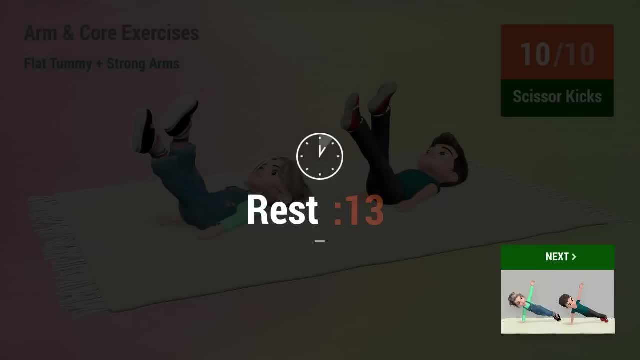 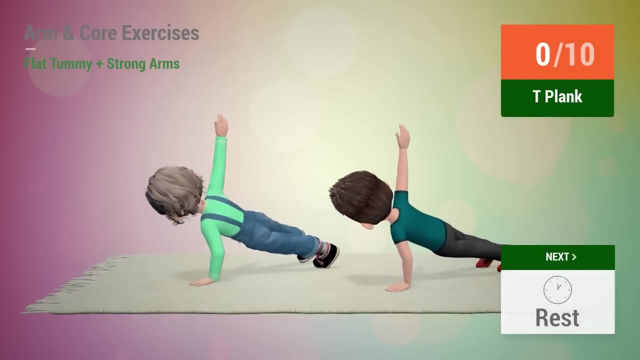 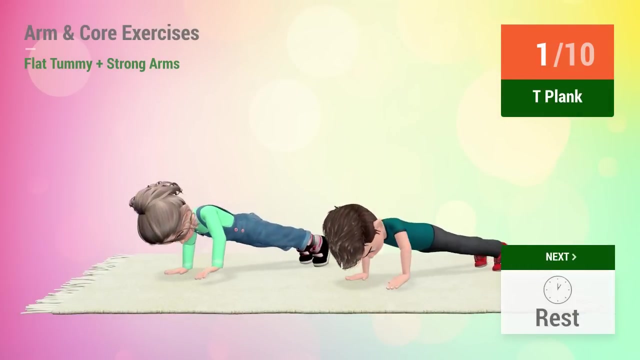 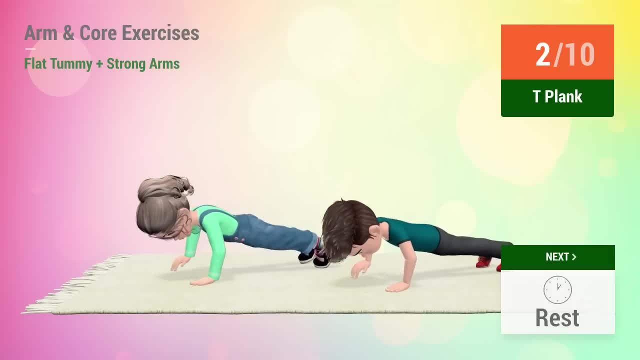 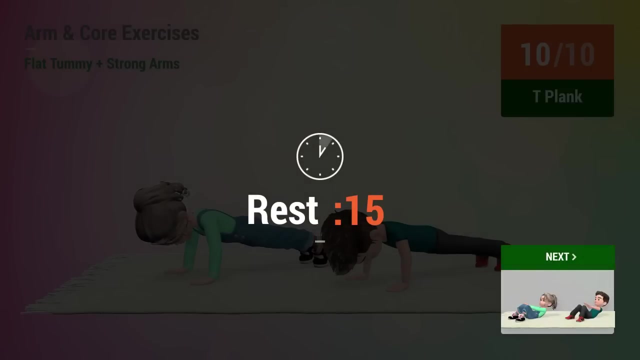 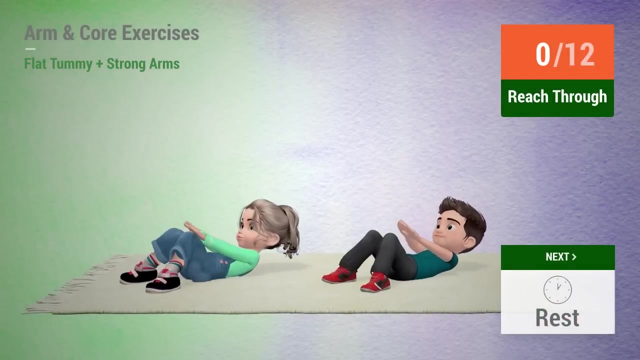 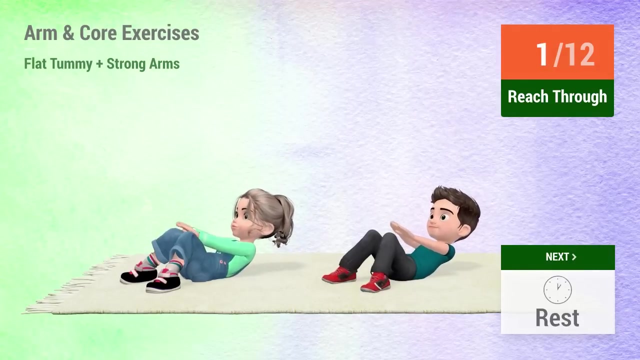 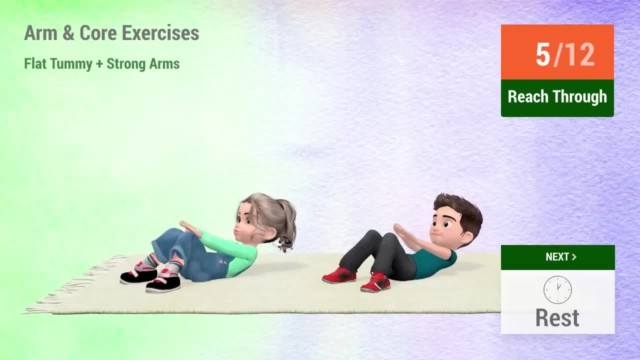 go one, two, three, four, five, six, seven, eight, nine, ten rest time. one, two, three, four, five, six, seven, eight, nine ten rest time 5,, 6,, 7,, 8,, 9,, 10,, 11,, 12. Rest time. 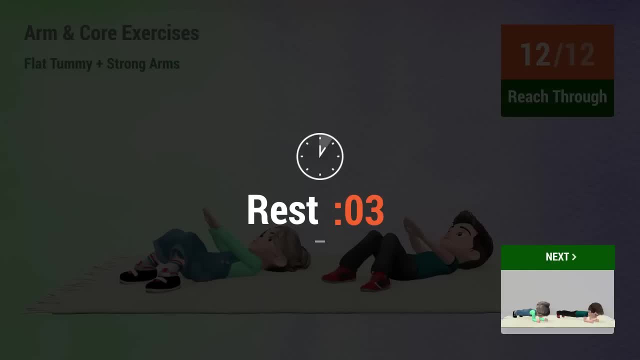 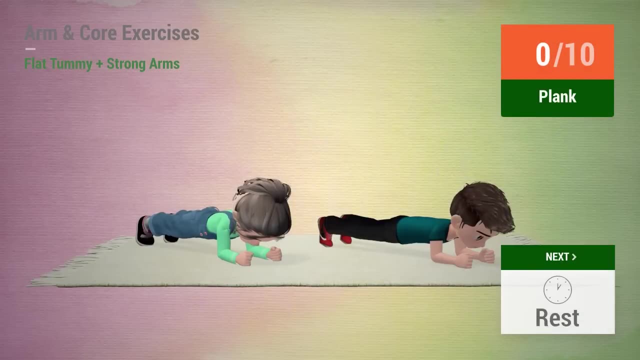 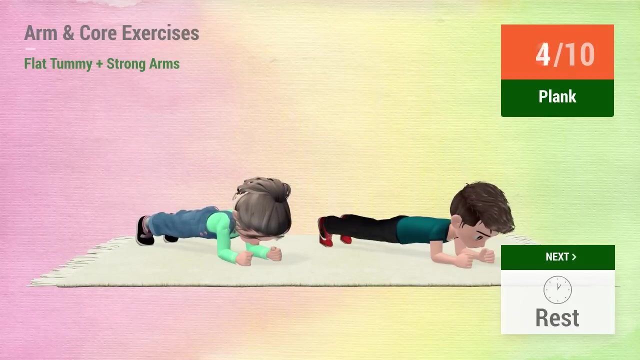 Up next plank In 5,, 4,, 3,, 2,, 1, go 1,, 2,, 3,, 4,, 5,, 6.. 7,, 8,, 9,, 10.. 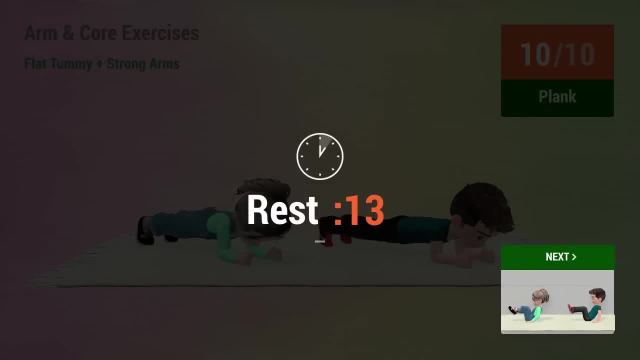 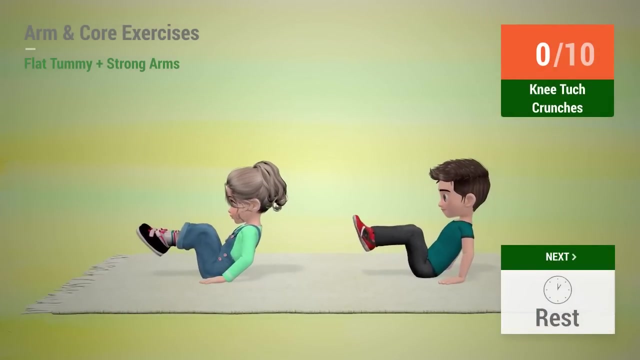 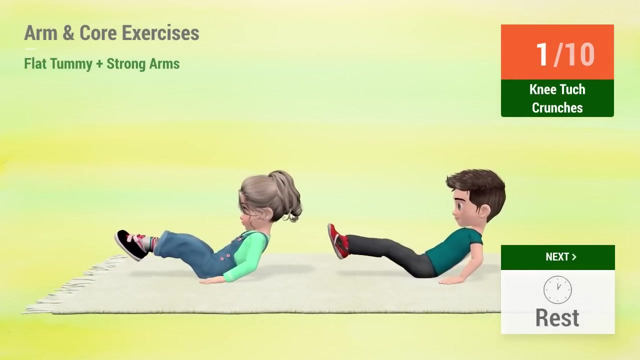 Rest time. Up next knee, tuck crunches In 5,, 4,, 3,, 2, 1, go 1, 2,, 3,, 4,, 5,, 6,, 7,, 8,, 9, 10.. 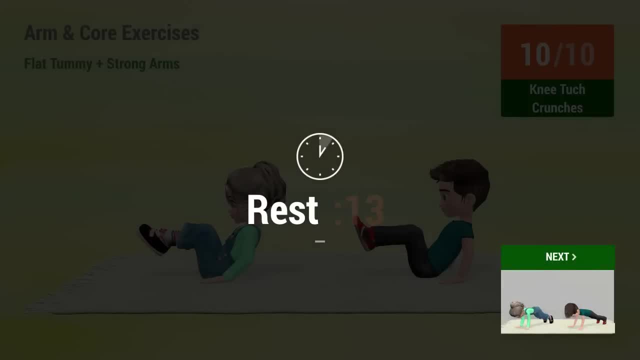 Rest time. Up next plank In 5,, 4,, 3,, 2, 1, go 1,, 2,, 3,, 4,, 5,, 6,, 7,, 8,, 9,, 10.. 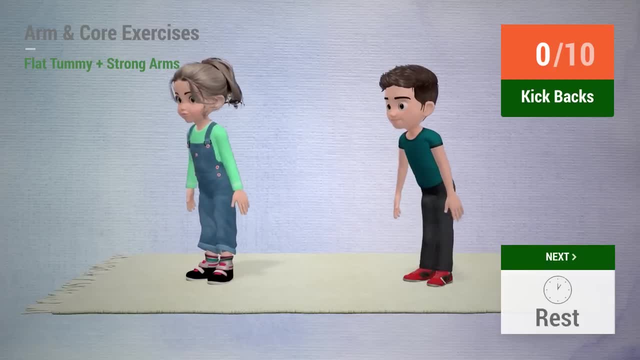 Rest time In 5,, 4,, 3,, 2,, 1, go 1,, 2,, 3,, 4,, 5,, 6,, 7,, 8,, 9,, 10.. 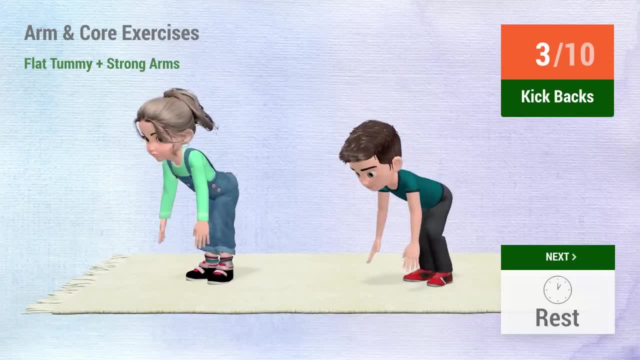 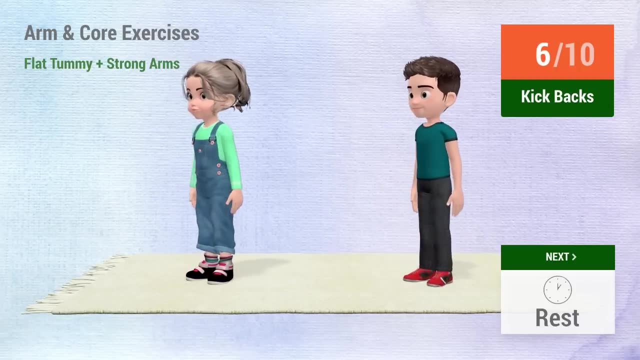 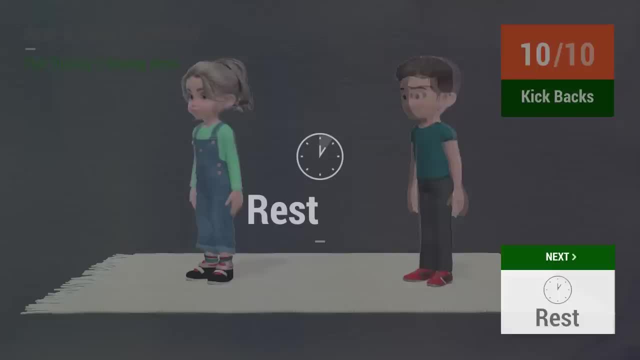 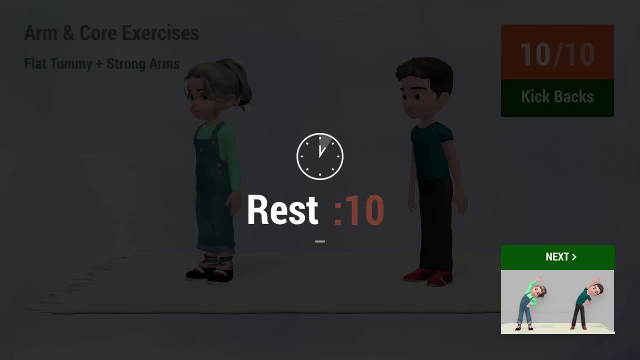 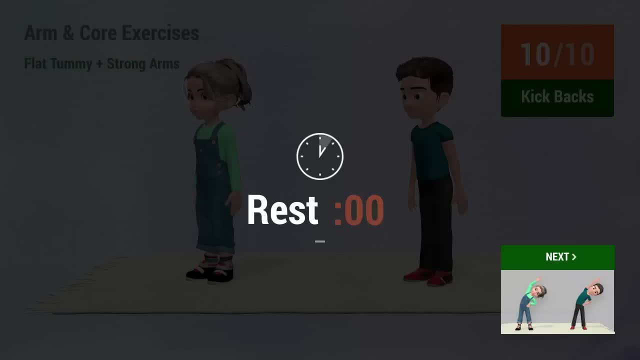 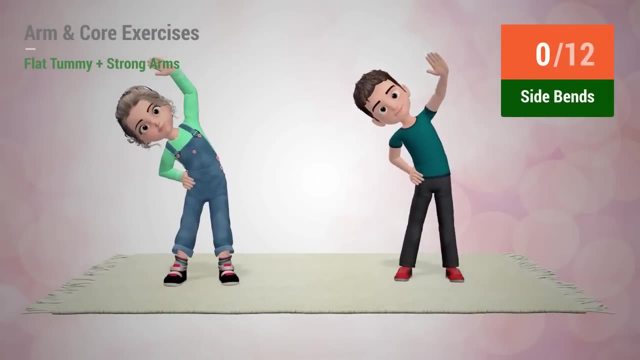 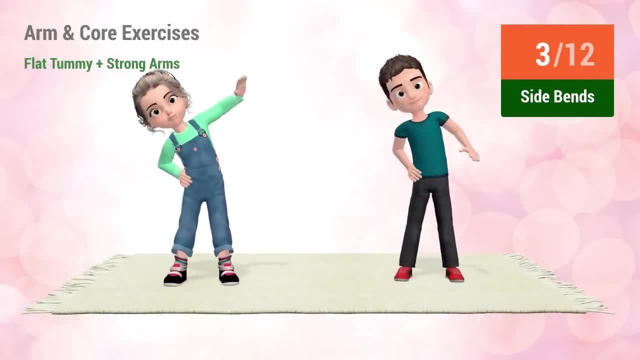